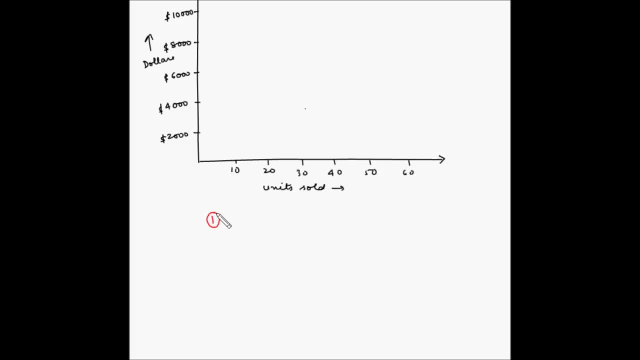 The first one is fixed cost, Second is the variable cost And the third is revenue. So let us understand how we can plot these three on this graph. Let us first take the fixed cost. Now we know that, by definition, fixed cost is the cost which does not vary by the volume. 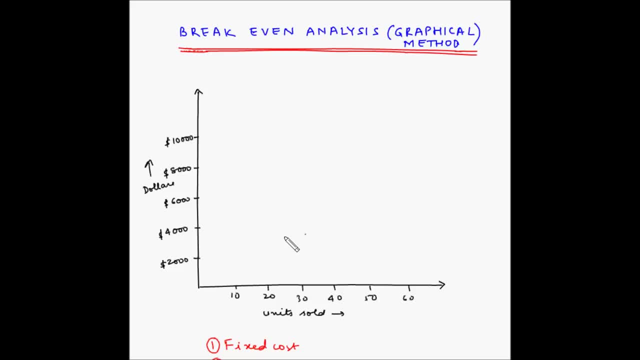 of production. So, irrespective of the number of units sold, the fixed cost will remain constant. So on the graph, if we have to plot the line basically, the cost will be the same if the number of units sold is 10,, 20,, 30,, 40, 50 or 60.. 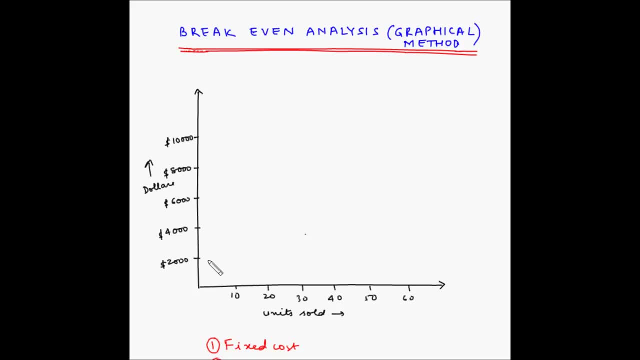 So what this gives us is a straight line. The fixed cost that we have is a straight line parallel to the x-axis. So let us draw that line. So let us say that the fixed cost is $2000.. So the line representing the fixed cost will be starting from $2000 and parallel to the x-axis. 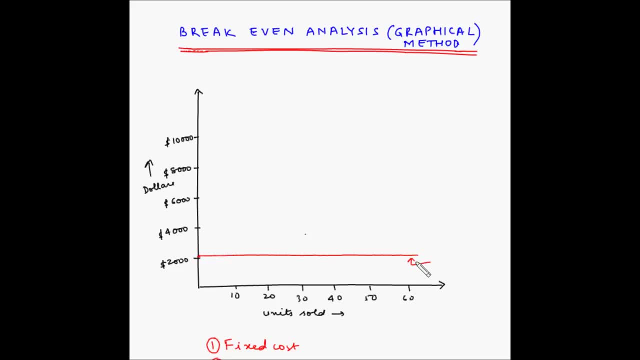 So this line here represents the fixed cost. so what this line means is that the fixed cost is $2,000, whether the number of units sold is 5, 10, 15, 20, up to any other number of units sold. now let's move to variable. 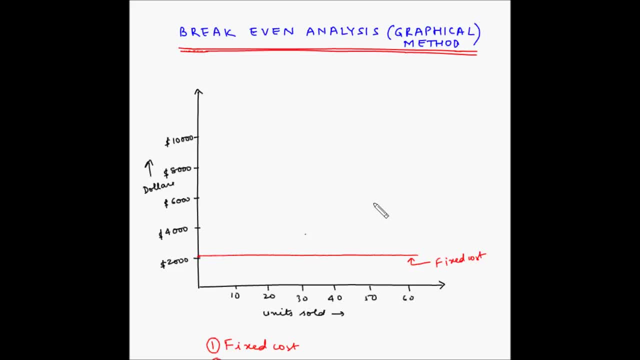 cost. so variable cost varies by the number of units sold. so if we have to plot the variable cost, so let's say this is the graph, with units sold on the x-axis and dollar amount on the y-axis. now if we don't produce anything, that is, if we have number of units as 0, then there is no cost. 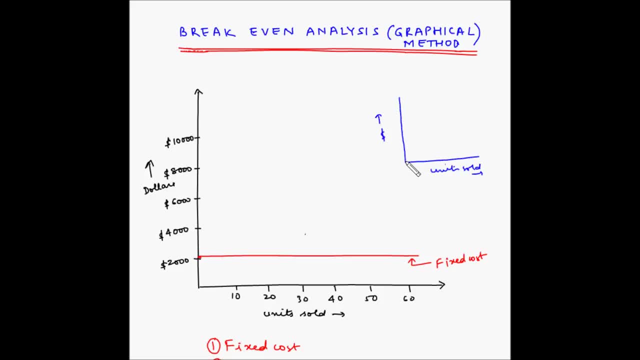 so there is no cost because we are not producing anything. so the line for variable cost will start from here and it will go like this: this will be representing the variable cost. the slope of this line will depend on the cost per unit. now again on this graph, the fixed cost will be a line like: 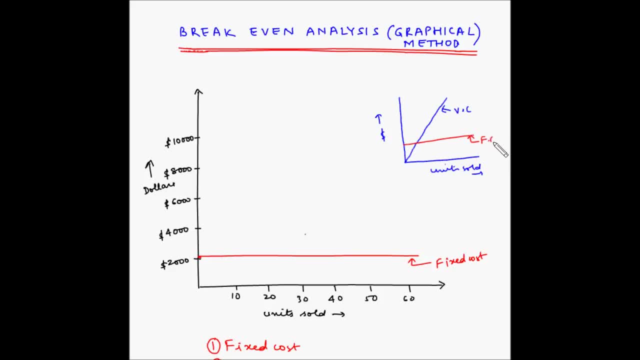 this. so this will represent the fixed cost and the variable cost will be the variable cost. so now if we add the two, the variable cost and the fixed cost, then we get the total cost. so if we have to draw the line for total cost on this graph, basically at this point when the number 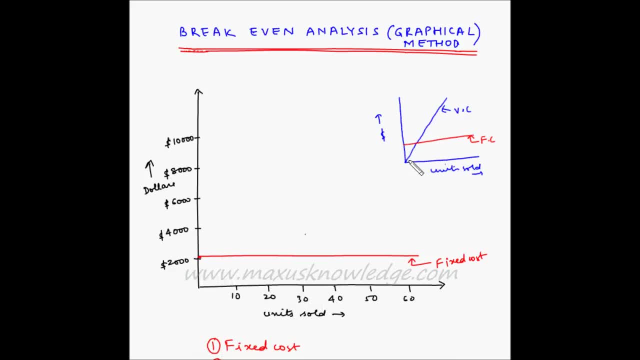 of units sold is 0, the variable cost is also 0, while there is a certain amount of fixed cost. so the total cost will start from here and we'll go like this. so this line will represent the total cost and basically on this total cost line at any point. 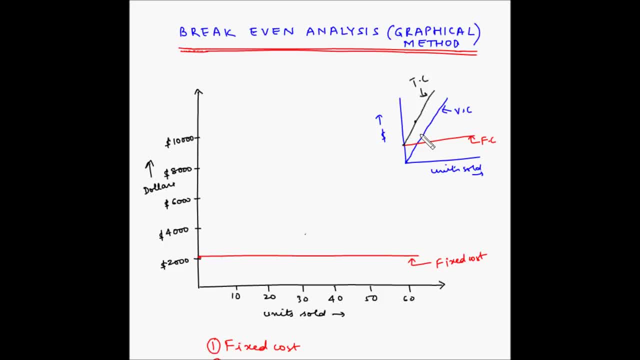 let's say this point: the total cost is the addition of the variable cost and the fixed cost at that number of units sold. so let's use this concept to draw the line for total cost on this main graph. so, as mentioned earlier, since the variable cost at 0 units is 0, however, fixed cost is 2000, so the total cost will start from 2000 and then as we 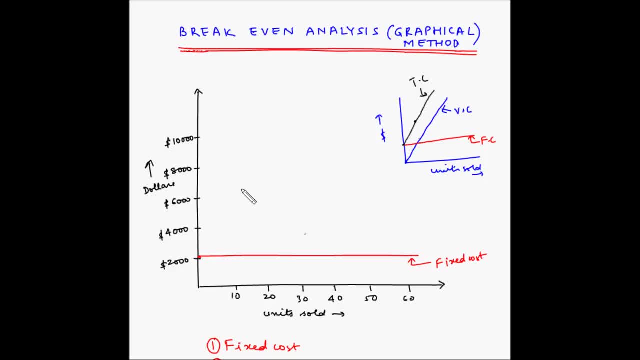 keep on adding the variable cost to the fixed cost, we will get the line for our total cost. now let's say that the variable cost is equal to 120 dollars per unit. so at the point where number of units is 40, let's find out the total variable cost. so if quantity 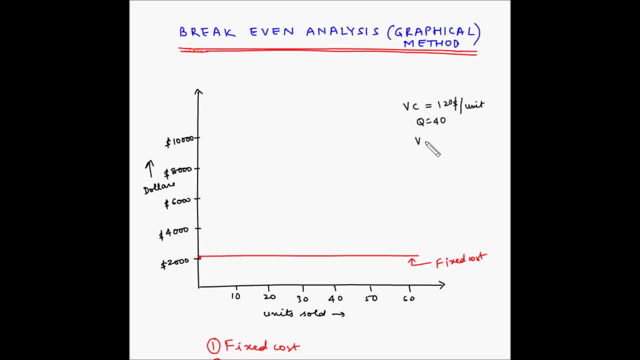 is equal to 40. the total variable cost is equal to 120 multiplied by 40.. 12 fours are 48, so 4800 dollars is the variable cost at 40 units. so for drawing the line for total cost, we already have one point, which is here at two thousand. 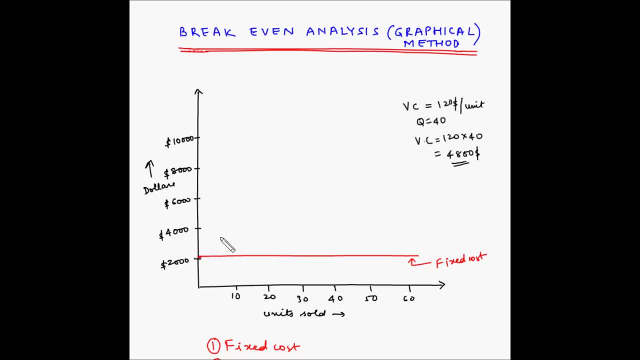 dollars. intercepting at the y-axis. and the second point is: at 40 units the variable cost is 4800 and if we add to this amount the fixed cost, so total cost will be equal to 4800, which is the variable cost plus fixed cost, which is two thousand. so this becomes 6800 dollars. so the second point. 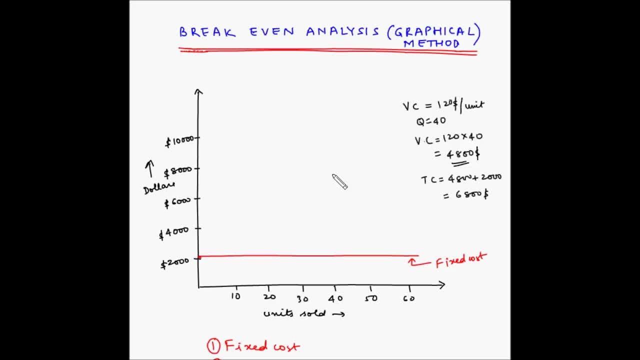 is 40 and 6800. let's say it is here somewhere. so with these two points let's draw the line for total cost. so this line here represents the total cost. now the third line which we have to draw is for revenue. let's say that each unit is being sold at a selling price of 200 dollars per unit. 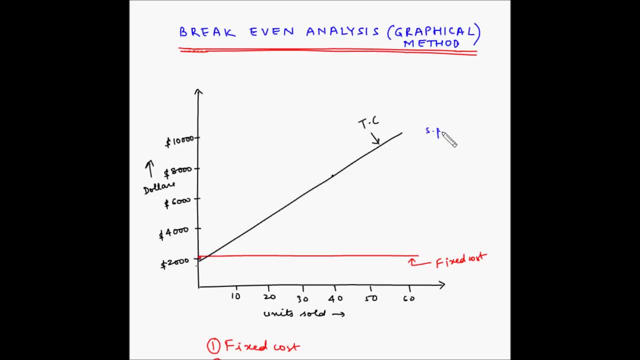 so selling price is two hundred dollars per unit. so at a point where zero units are sold, the total revenue will be zero. now let's find out the total revenue at a point where 40 units are sold. so the total revenue will be equal to 200 multiplied by 40, which is equal to four, twos are eight. 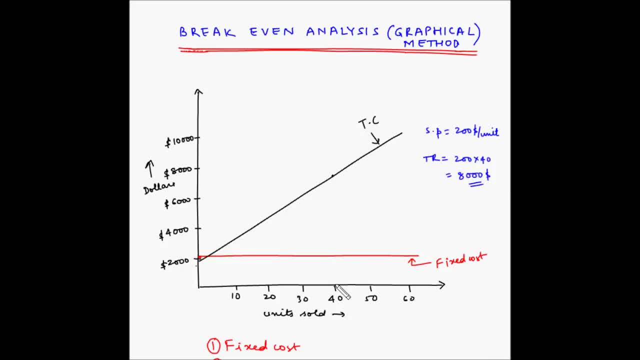 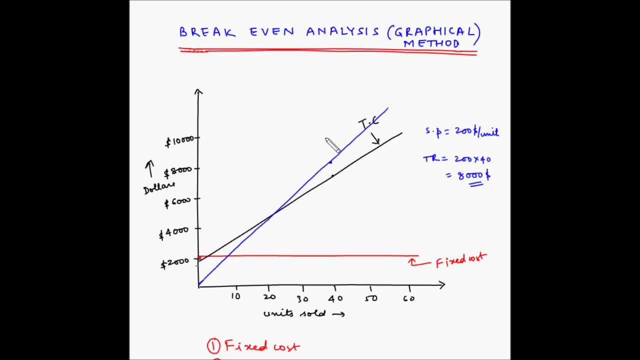 so this represents the total revenue. so on this graph, the point at which the total revenue is equal to the total cost is this point here where both of them are intersecting each other, and this point is known as the break-even point. so this is the break-even point. 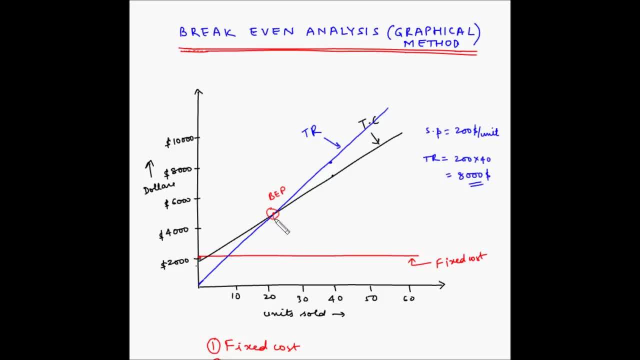 now, if we draw a line parallel to the y-axis touching the x-axis, then the point here on the x-axis will represent the break-even point in terms of units sold. and if we draw a line parallel to the x-axis touching the y-axis, like this, then this point here will represent the 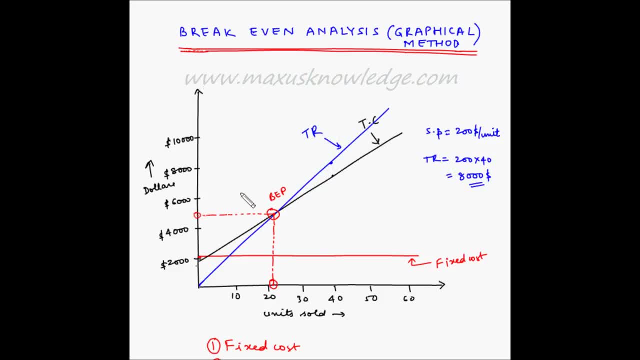 break-even point in terms of dollars. you now again, since this graph is not on scale, so these numbers may not be accurate, but these are representative of how you can actually achieve the break-even point using graphical method. now this region here below the break-even point represents the area of loss. 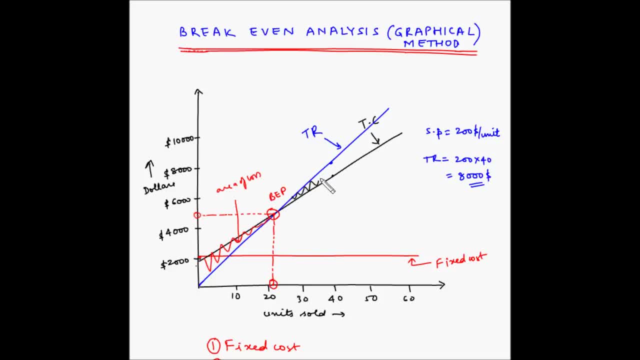 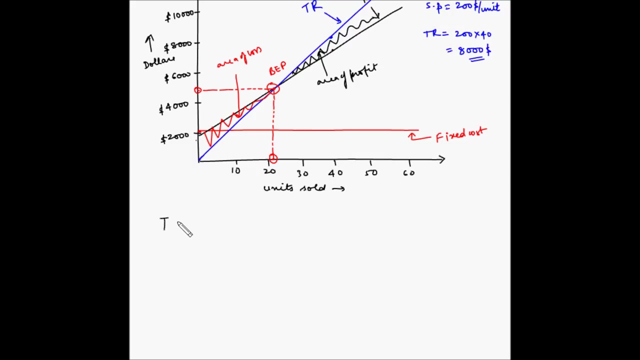 while this region here above the break-even point, represents the area of profit. now one question that comes to mind is that how do we know that these lines are linear or straight in nature? so let's take the example of the total cost line to understand this. now we know that the total cost is equal to the fixed cost plus the variable cost. 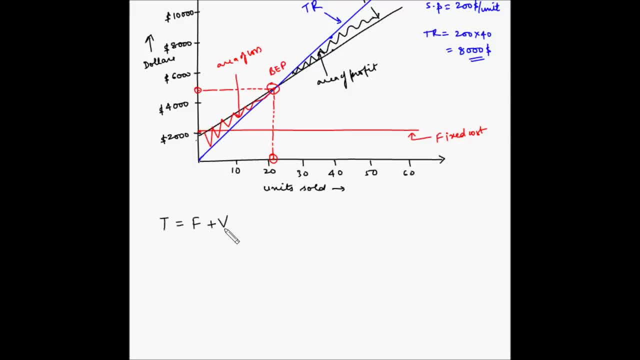 And the variable cost is equal to the number of units multiplied by the unit variable cost. So T is equal to F plus, let us say, Q is the number of units and small c represents the unit variable cost. Now we know that the formula for a straight line is: Y is equal to MX plus C. 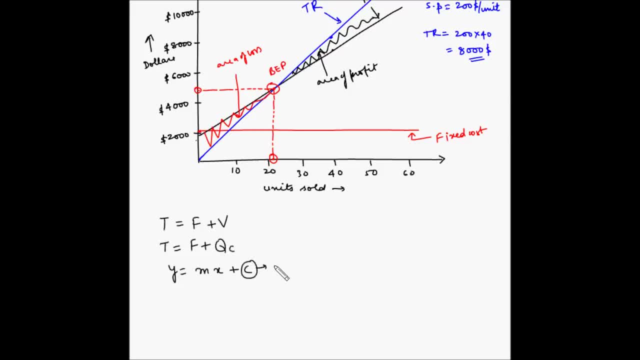 Here C is a constant, that is a numerical value, M represents the slope of the line and X is the variable. So in this equation for a straight line, C is the point where the line intercepts on the Y axis. So now let us put the equation for total cost in terms of a straight line. 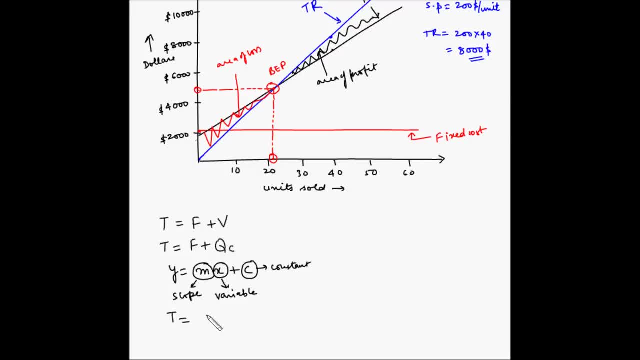 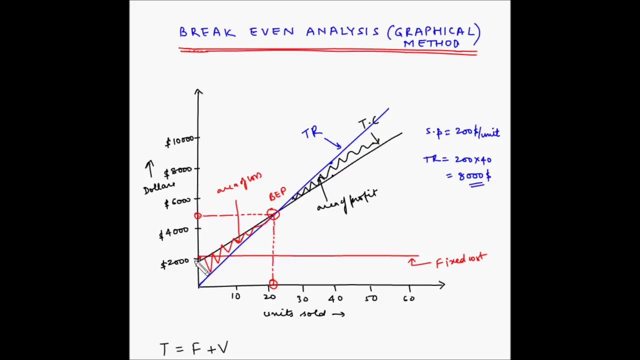 So we get: T is equal to CQ plus F. So here F is the constant or the Y intercept. So if we look at the at the graph, the total cost line intercepts the y axis at a point which is equal to the fixed cost. 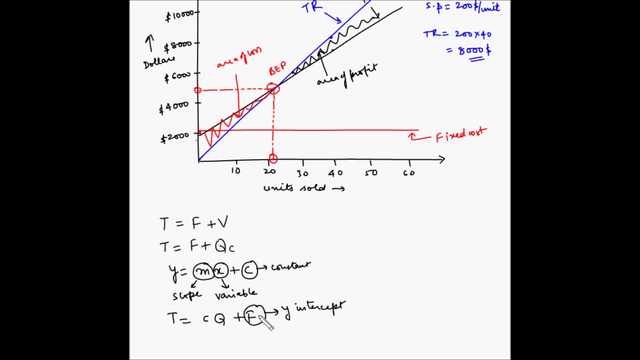 which is in our case two thousand dollars. so f is the y intercept, or the constant small c represents the slope. so basically, the unit cost of the product determines the slope of the total cost line and q is the variable. now let's do the same thing for the total revenue line. 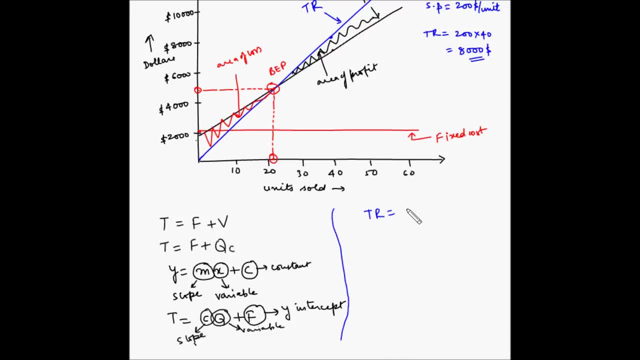 now we know that total revenue is equal to the quantity of units sold multiplied by the unit selling price. now the equation for a straight line is: y is equal to mx plus c. so if you try to put the equation of total revenue in this terms, we get: 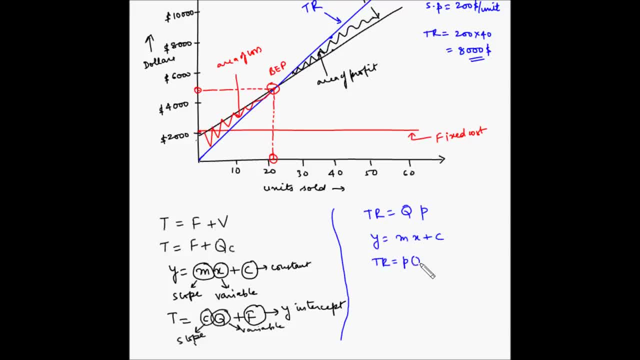 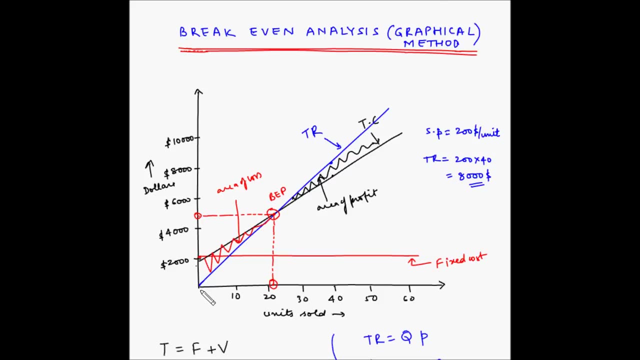 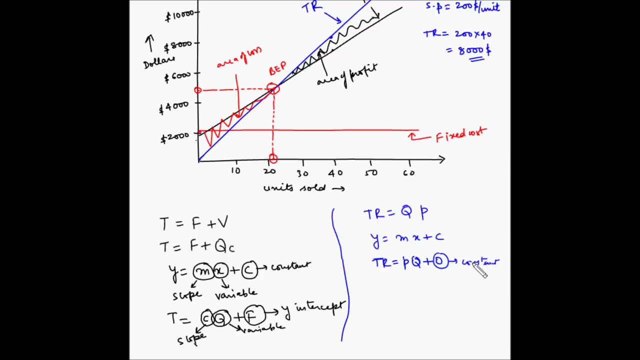 total revenue is equal to p multiplied by q plus zero. now, as we know, c is the point at which the line tercepts the y axis, and the total revenue line intercepts the y-axis at 0. so this is the constant. in this case, P is the unit selling price.